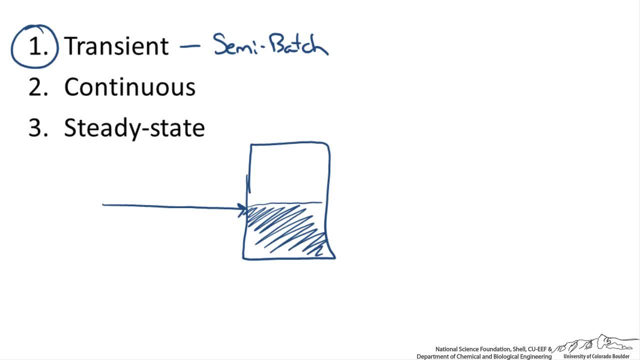 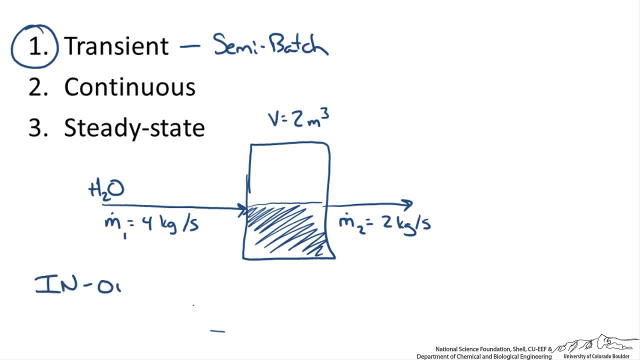 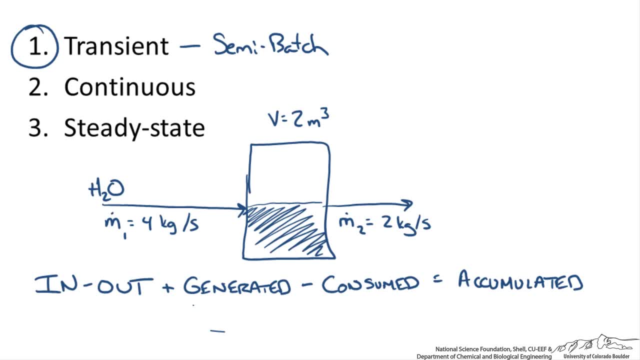 reactions, but for most things that you are going to see, let's just say that mass cannot be generated or consumed. We also know that if there is no reaction taking place, then a species like water cannot be generated or consumed. So it all depends on how we decide. 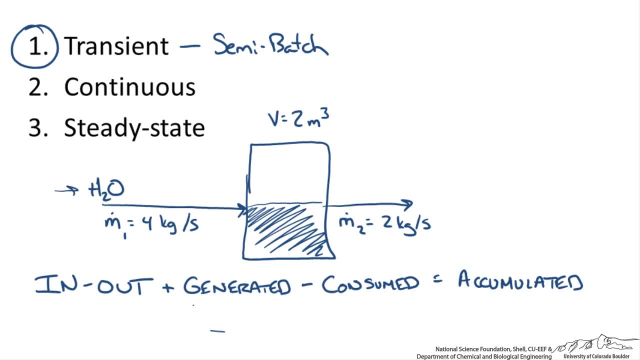 to do this process. We could either write a species balance for water or a mass balance for water. In this case they are the same thing. If we had multiple components, then we could write different species balances and we could see some other examples that will do that. So, very generally, because we don't have a reaction, and since we are working, 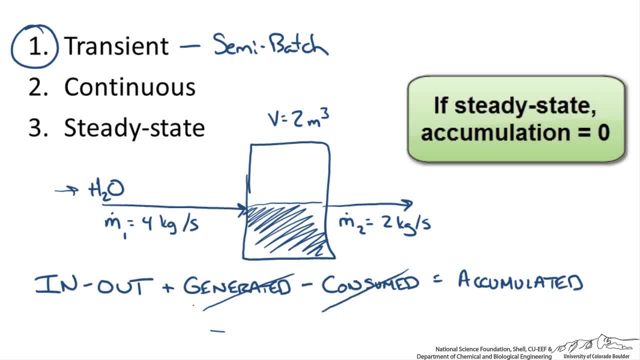 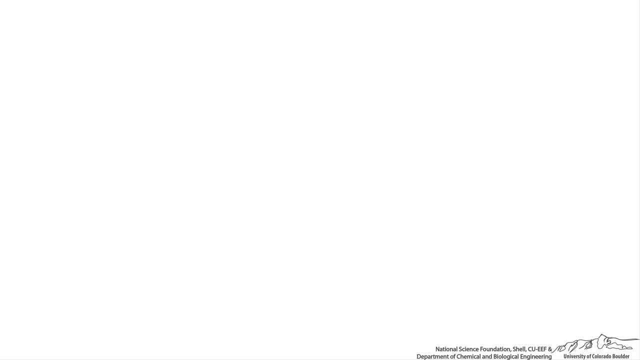 on a mass scale, we are going to say that there is no generation or consumption. So our balance here comes down to n-out equals accumulated. So if we want to figure out how long it takes to get this tank filled up, let's go ahead and go back to our material balance. We know 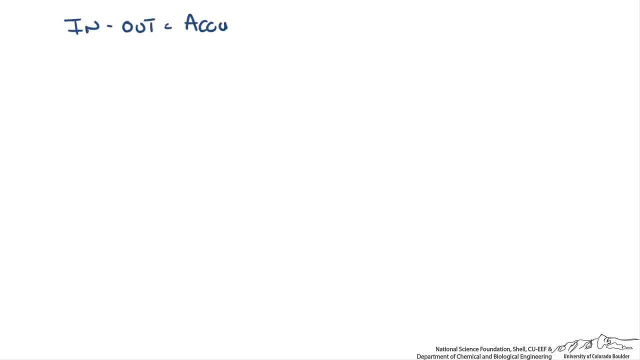 that n-out equals accumulated. I will just abbreviate that To redraw my picture really quick. So here is our schematic and our mass balance. So at this point we can pretty much just fill in some numbers. That would be the next logical step. So if we write it again, 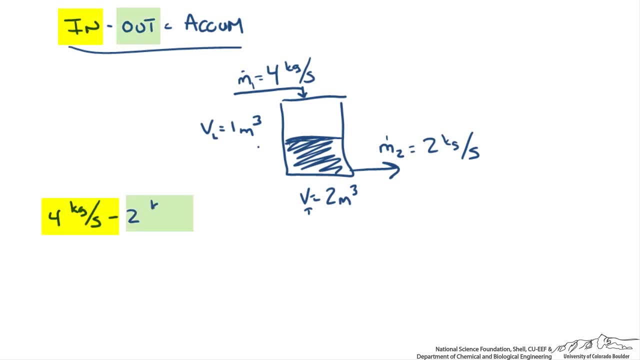 make sure we have the units down: 4 minus 2 kilograms per second. out has to be the accumulation. So the accumulation is going to be 2 kilograms per second. Now, if we convert this to a volume, we are going to need some kind of conversion factor, The conversion factor from volume. 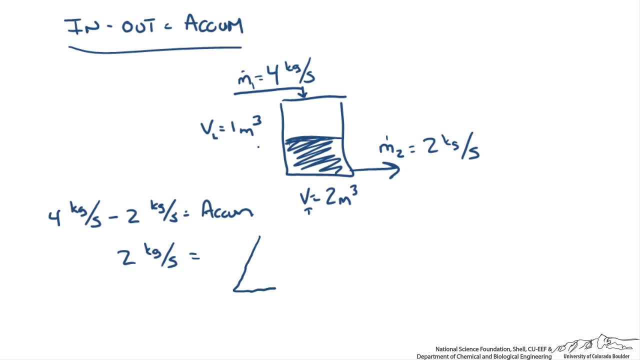 to mass. Mass is density. A nice way to remember this. I always kind of go back to a triangle. We know that density has to equal mass to volume. So depending on which one you need, you cover that up and you can do the calculation with what you have. So in this case we have mass. 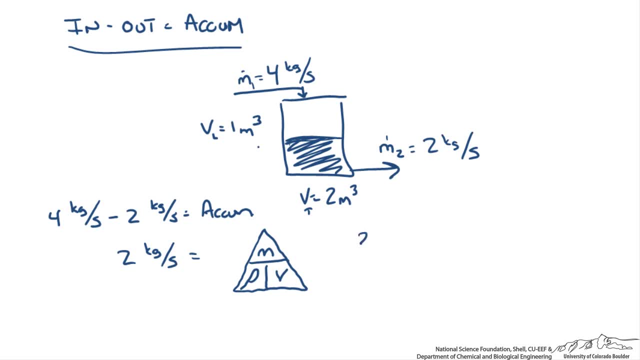 We need volume. So we are going to take mass and divide by density. So 2 kilograms per second divided by the density of water, which is 1 kilogram per liter, is going to give us 2 liters per second. However, we are not working with liters. we are working. 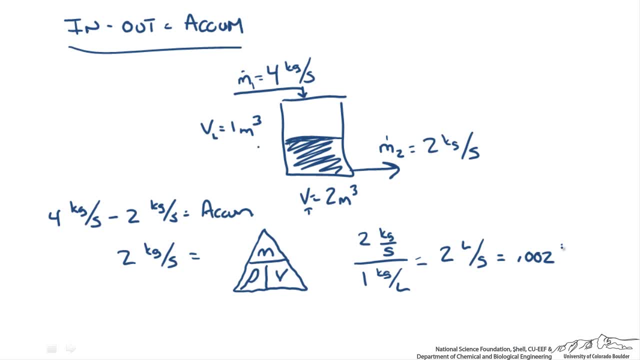 with meters cubed. So this is going to be 0.002 meters cubed per second, Because there is 1000 liters per meter cubed and we are going to divide by that to cancel out our liters and get meters cubed on top, We have 0.002 meters cubed per second. We know that. 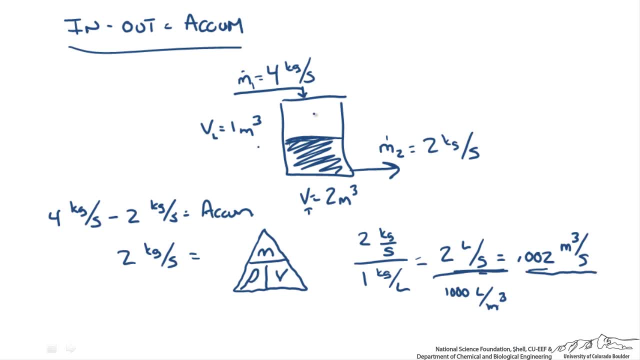 we need to fill 1 meter cubed until this tank is full. Now that is the empty space. That's, that is the empty space. So in this case we could write an integral balance where volume is going to be the volumetric flow rate times some time interval. In this case we write: 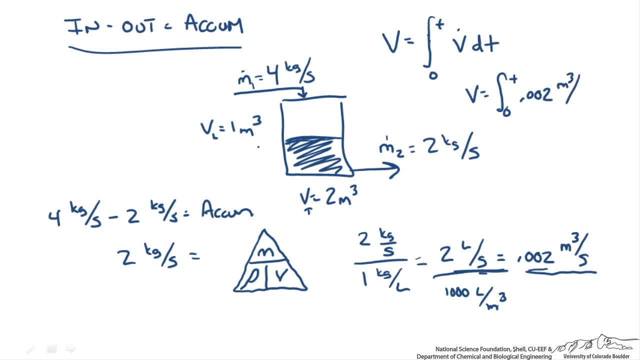 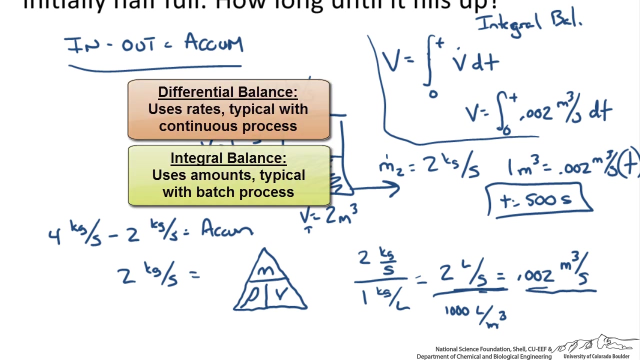 this out: 0.002 meters cubed per second dt. and we know 1 meter cubed equals 0.002 meters cubed per second times t. So t is going to equal 500 seconds. So that is what is called an integral balance. If we were trying to figure out the rate instead, then we would.